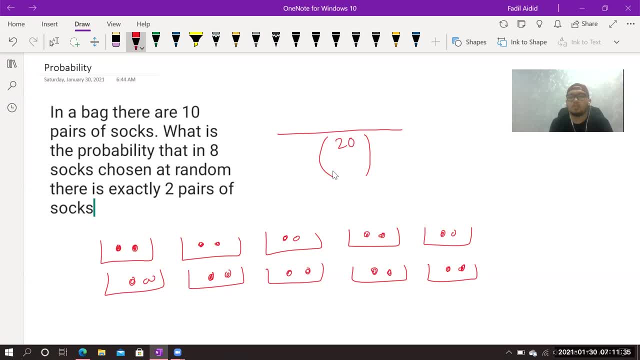 This is the total sample space, Total outcomes, And then for the numerator is what we want. So for the numerator: we want exactly 2 pairs of socks. So we want exactly 2 pairs is 10, not 20 again because we want to see from the pairs angle point of view. okay, so the total. 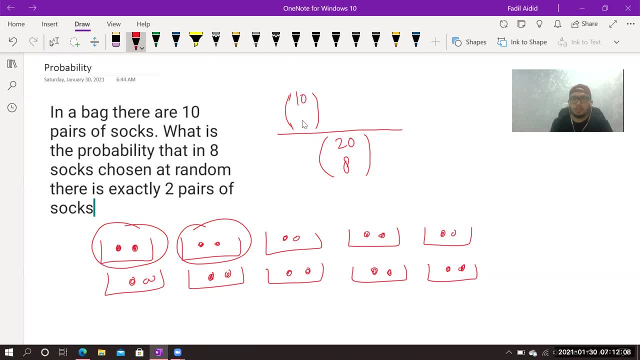 pairs. now we're talking about pairs, so 10, and then we want to get exactly two, so that means the remaining socks. the other four socks must be different, right, because you want to get exactly two pairs, so only four socks. that exactly the same, okay. for example, this the first. 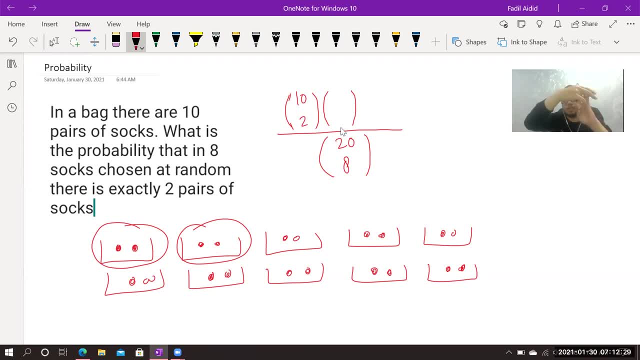 two socks is from the first pair and then the other sock is from the second pair, for example. so that means the other remaining. the remaining must be different, so must be select from each of this box. okay, so for example, for this we need to select only one. we cannot select two from this. 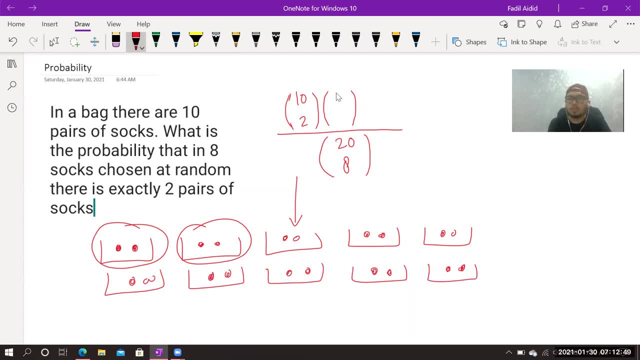 single box for the remaining. yeah, so that means the rest is just eight pairs, and then we choose four, four, four. but how can you know that? i mean, if we only write this, it is not guaranteed that these four remaining socks is different each of this. so to guarantee that we know that each of this box has two object, right, so that means we only 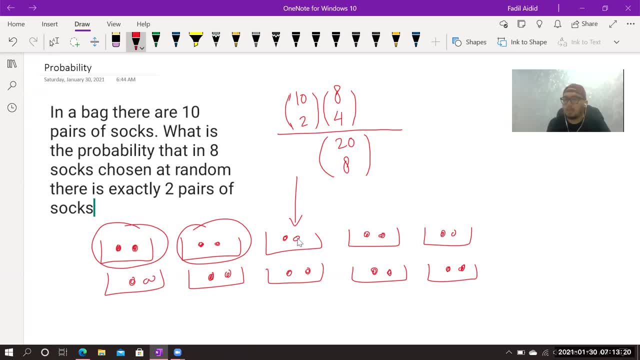 want to get one of these two object. so that means this is like a combination of one from two. this is like the choosing way. okay, the the way of choosing for the remaining socks. okay, so two from- i mean sorry, one from two socks, okay, we. and then we know that the remaining socks is only four, so we need to make 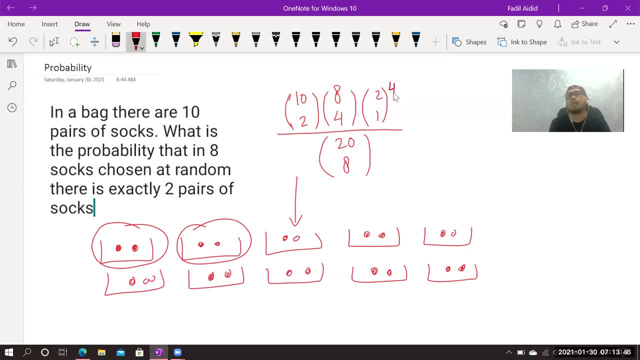 it power of four. so this is that guarantee that the remaining four socks is different, like it's not the same. it selects from each different box, not from the same box. okay, so this is how you answer this problem. okay, let's say the question is changed like: still 10 socks and then still, we want to get eight. we want to choose eight socks.